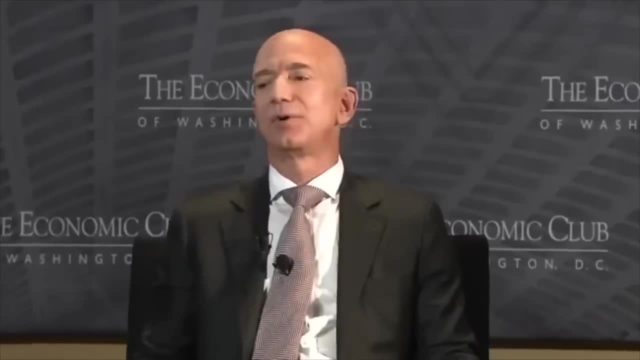 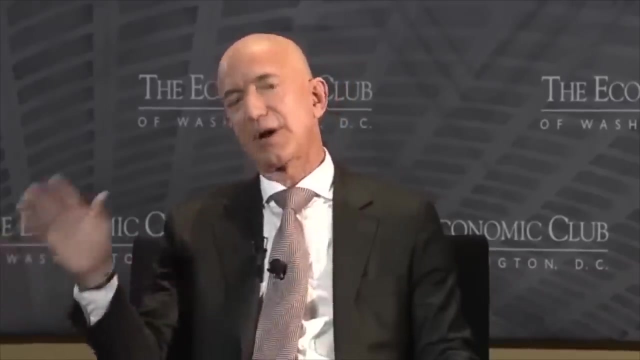 Because I wanted to be a theoretical physicist and so I went to Princeton and I was a really good student, as I pointed out already. I got A pluses on almost everything. I was in the honors physics track, which starts out with 100 students, and by the time you get 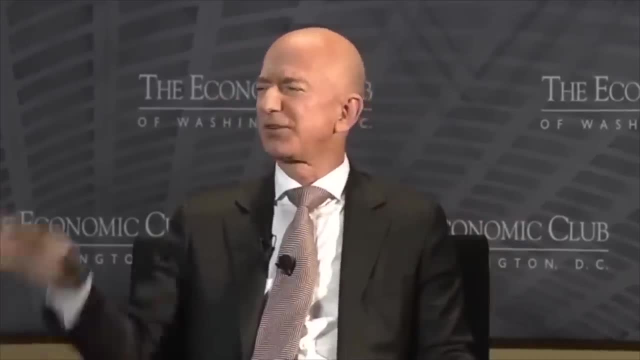 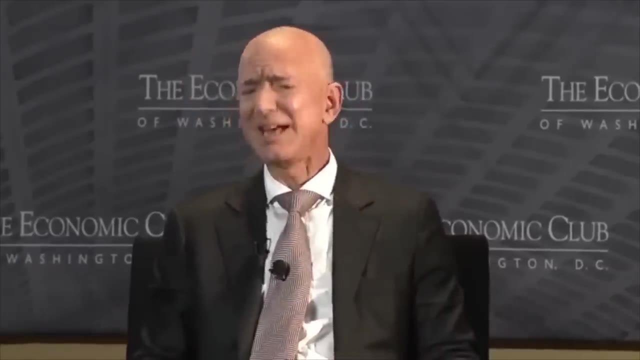 to quantum mechanics. it's like 30. So I'm in quantum mechanics- I think this is like junior year- and I've also been taking a bunch of computer science classes and electrical engineering classes, which I'm also enjoying, and I can't solve this partial differential. 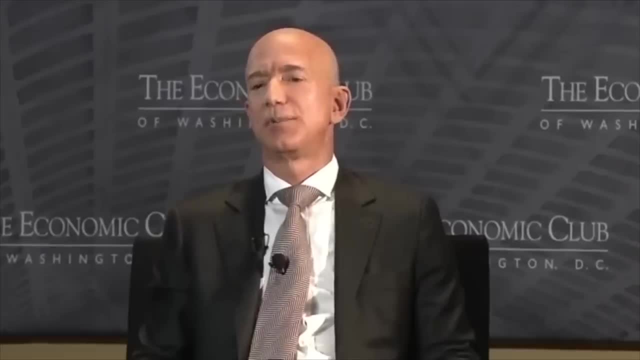 equation. It's really really hard and I've been studying with my roommate, Joe, who also is really good at math, and the two of us worked on this one homework problem for three hours and got nowhere and we finally said we looked up at each other over the table. 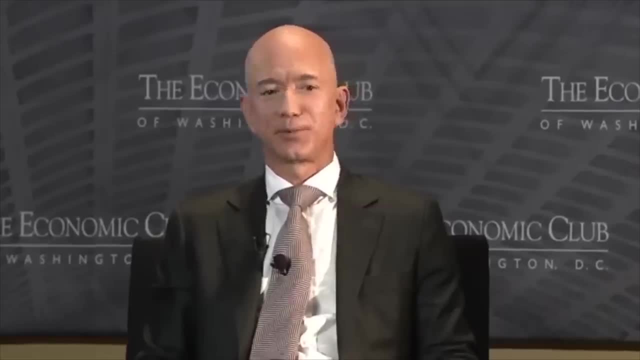 at the same moment and we said yo Santa, Because yo Santa Santa was the smartest guy at Princeton. and we went to yo Santa's room and he was Sri Lankan and in the Facebook, which was an actual paper book at that time, his name. 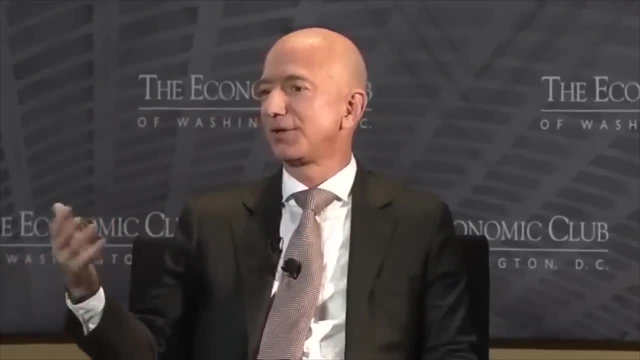 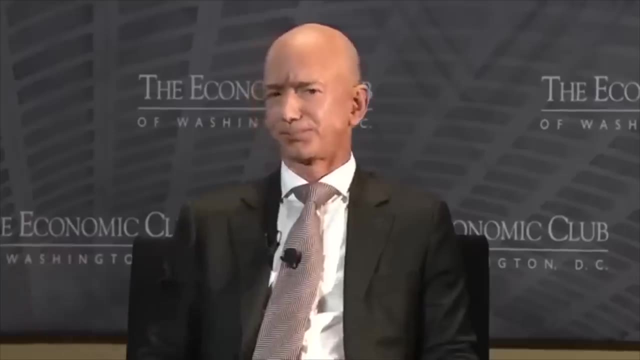 was three lines long because I guess in Sri Lanka when you do something good for the king, they give you an extra syllable on your name, And so he had a super long last name, the most humble, wonderful guy. and we show him this problem and he looks at it and 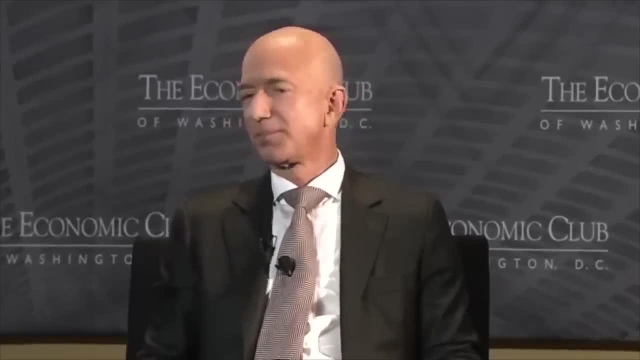 he stares at it for a while and he says: cosine. And I'm like: what do you mean? He's like: that's the answer. And I'm like that's the answer. And he's like: yeah, let me show. 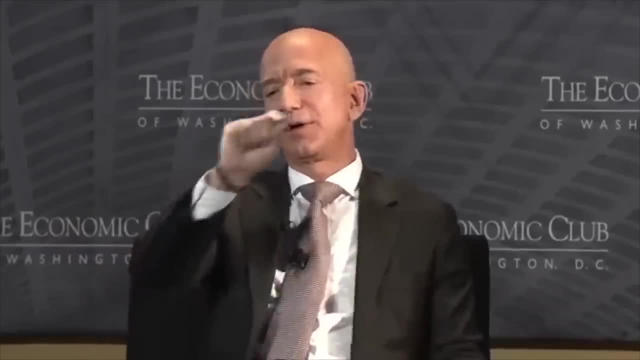 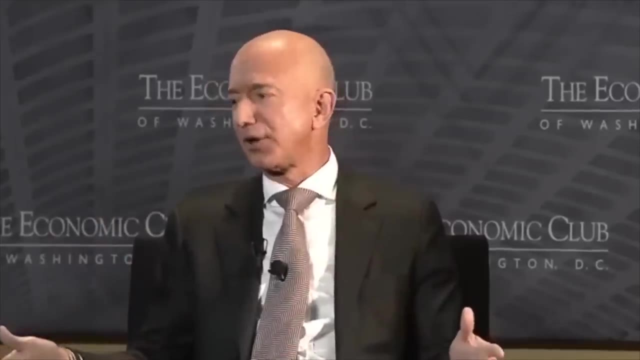 you. So he brings us into his room, he sits us down, he writes out three pages of detailed algebra. everything crosses out and the answer is cosine. And I said: listen, yo Santa, did you just do that in your head? And he said no, that would be impossible. 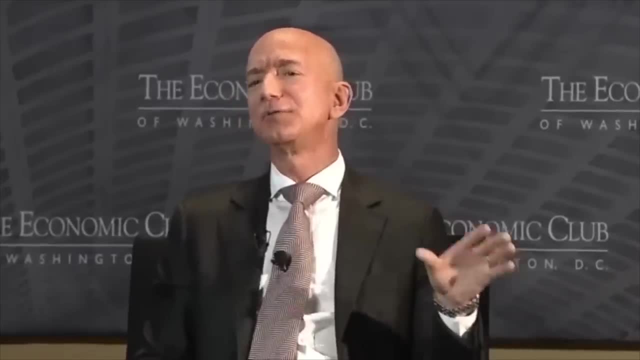 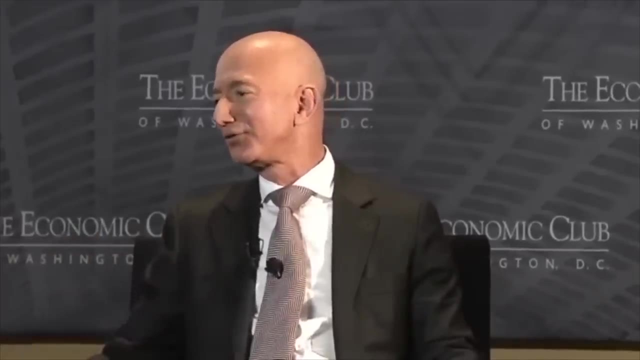 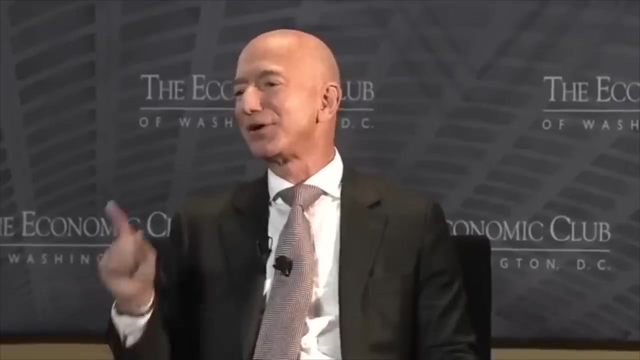 Three years ago I solved a very similar problem and I was able to map this problem onto that problem and then it was immediately obvious that the answer was cosine And I. that was an important moment for me, because that was the very moment when I realized I was never. going to be a great theoretical physicist.